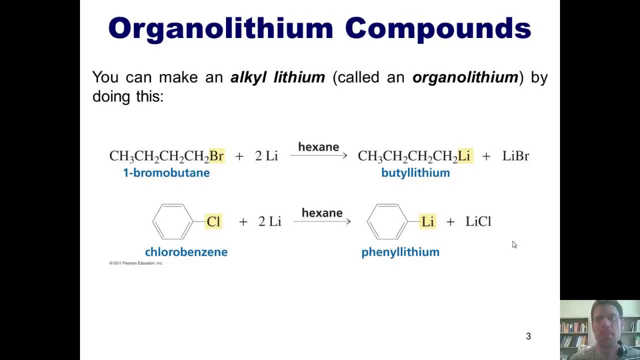 two equivalents of lithium and generate this molecule, phenyl lithium. Now you might ask: why in the world would I ever want to make an alkyl lithium or organolithium compound? Don't worry, I'll show you that momentarily. 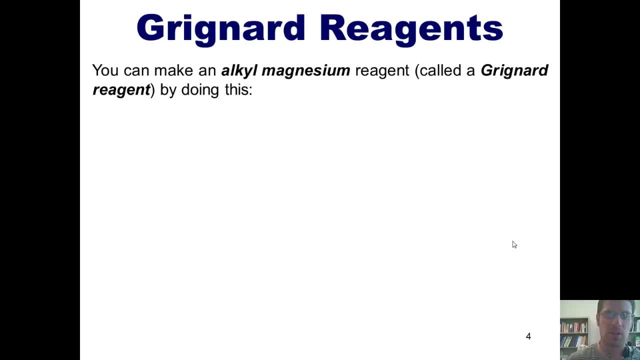 But before I do, I want to also show you how to make this type of reagent. You can make an alkyl magnesium reagent, which is also called a Grignard reagent. by doing this, You take any type of alkyl halide, such as an alkyl bromide shown here. 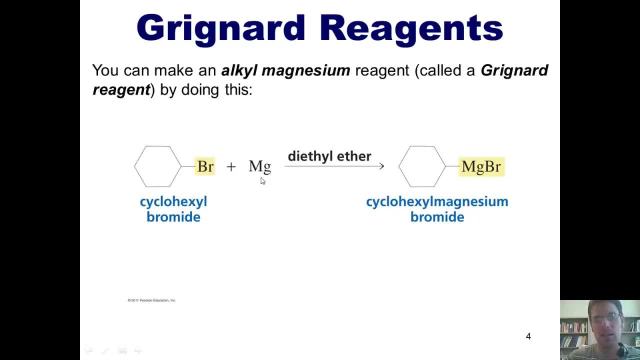 react it with magnesium metal and what ends up happening is the metal inserts itself between the hydrocarbon chain and the bromine. This type of molecule is called a Grignard reagent. Here's another example. I've got this molecule which is called vinyl bromide. 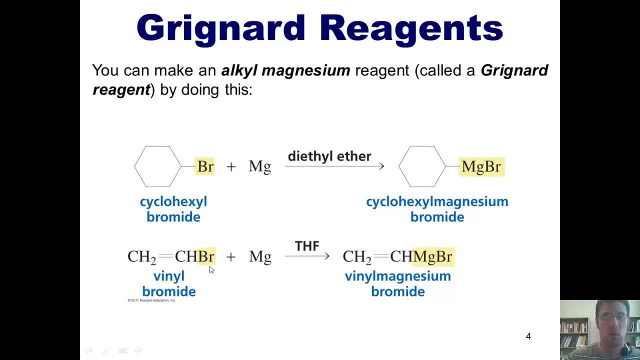 Once again, it's a bromine attached to a carbon, but this could also work with a chlorine or an iodine, And I react it with magnesium. The magnesium inserts itself between the carbon and the halogen. Once again, these types of reagents are called Grignard reagents. 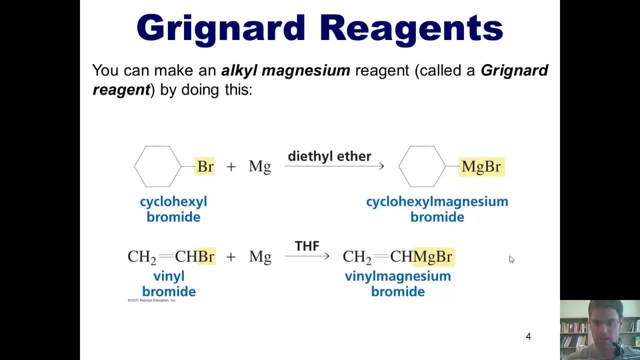 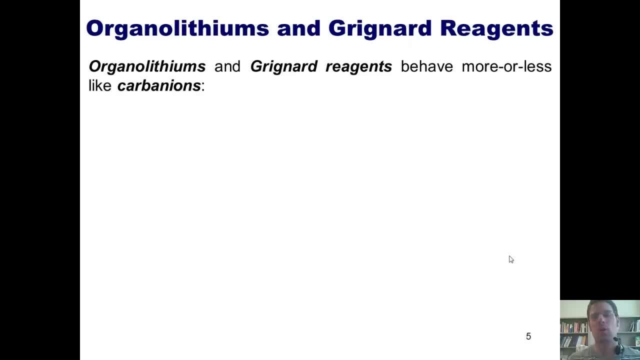 And yes, that is pronounced Grignard, not Grignard Ugh. So what in the world can we do with these types of reagents? Well, organolithiums and Grignard reagents behave more or less like carbanions. 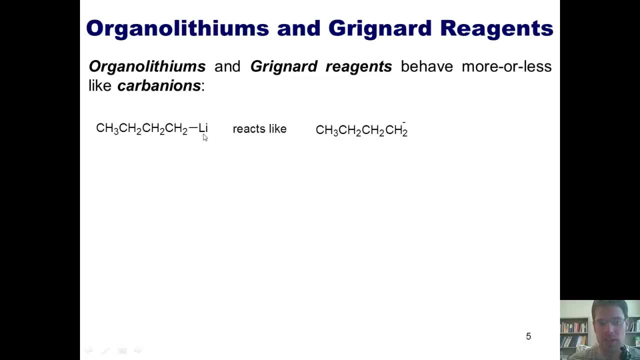 For example, if I've got this type of molecule stuck to a lithium which is called butyllithium, it essentially behaves as if there's a negative charge on the carbon that's bonded to the lithium. So it'd behave kind of like this molecule right here where there's a negative charge on this carbon. 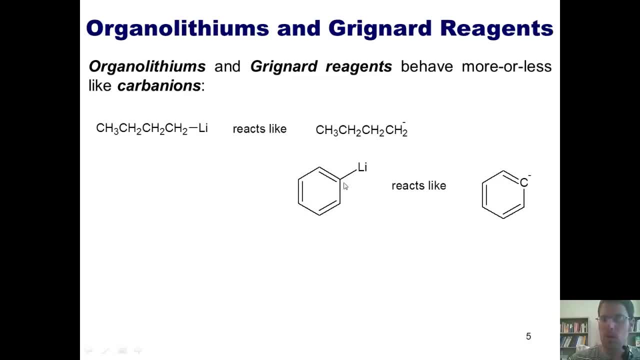 Similarly, phenolithium shown here would react more or less as if there were a negative charge on this carbon right here, as I've indicated here. Similarly, a Grignard reagent such as the one shown here behaves more or less as if there's a negative charge. 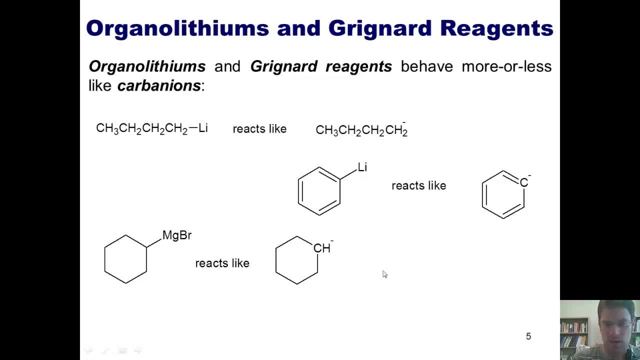 on this carbon, the one bonded to the magnesium, as shown here And, in this example, vinyl magnesium bromide. it would behave more or less as if there were a negative charge on this carbon, the one that's bonded also to the magnesium. 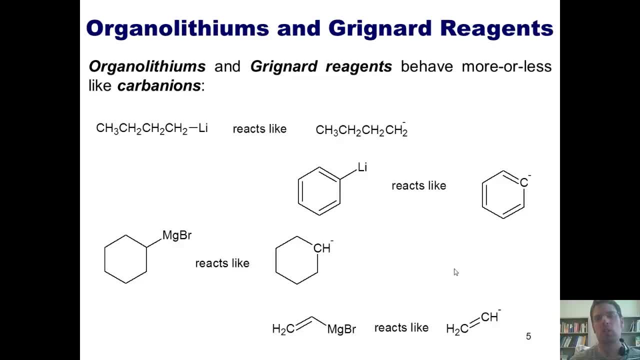 Now up to this point. we've traditionally talked about carbons as having partial positive charges, and the reason is because most of the reactions we've discussed- they're often bonded to halogens or oxygens or nitrogens or other elements that are more electronegative than the carbons themselves. 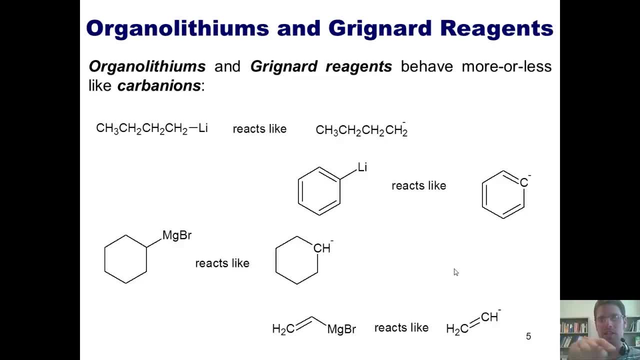 In these types of reagents- reagents in which I have a metal bonded to a carbon- you'll note that carbon is much more electronegative than the metal, So in these circumstances, the carbon is the guy who ends up hogging the electrons. 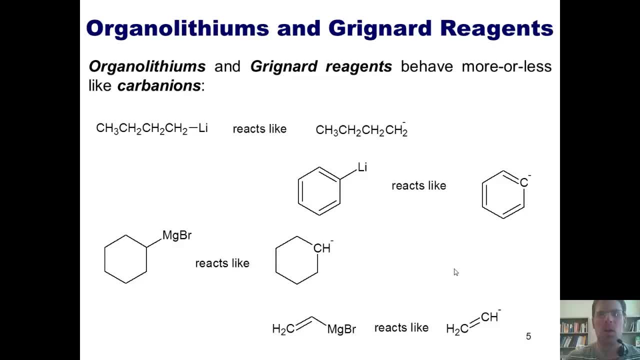 which once again makes him behave as if he were more or less like a carbanion, a negatively charged carbon. So you might wonder: why is that useful? Well, as it turns out, you can take a molecule such as methyl lithium, shown here. 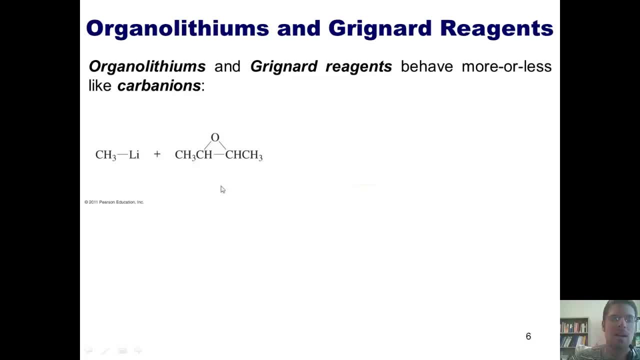 and react it with an epoxide, for example The methyl lithium, once again behaves as if there's a negative charge on this carbon. What that does, then, is that the negatively charged carbon comes in here and attacks, like a nucleophile, one of the two carbons in this epoxide. 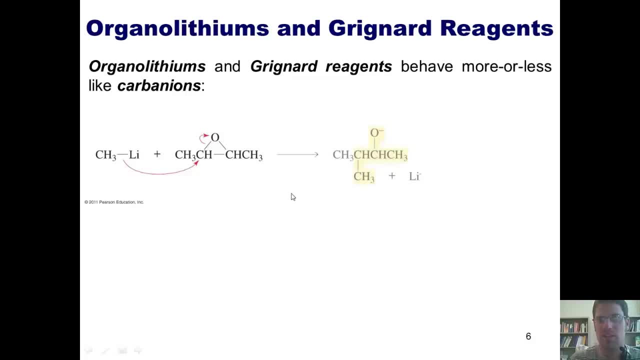 and pushes these electrons up onto the oxygen, Giving me this intermediate. This negatively charged oxygen can then be protonated by adding water or acid to give us this type of product. Once again, you can see that this alkyl group that was attached to the lithium 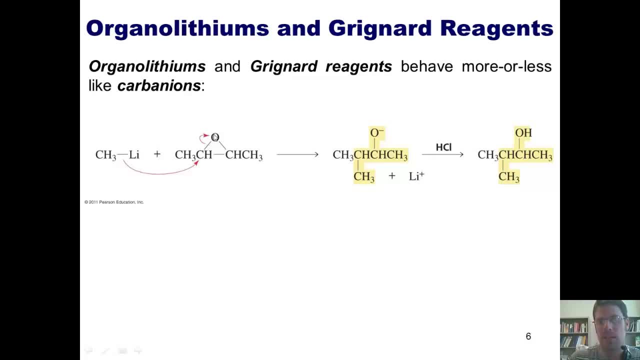 acts as a nucleophile to come right in here and pump these electrons up onto the oxygen. Similarly, if I take a Grignard reagent, it more or less reacts as if there were a negative charge on this carbon, the one that's bonded to the magnesium. 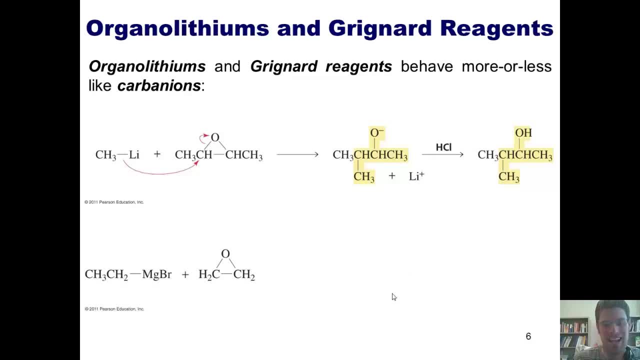 It then uses those electrons to mark and charge, as if it were a negatively charged carbon, into this carbon bound to the oxygen in our epoxide. pumping these electrons up onto the oxygen and giving me this intermediate, You'll notice that this ethyl group, the CH2CH3 group, 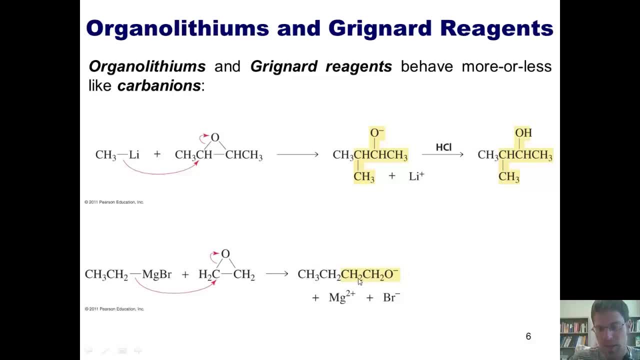 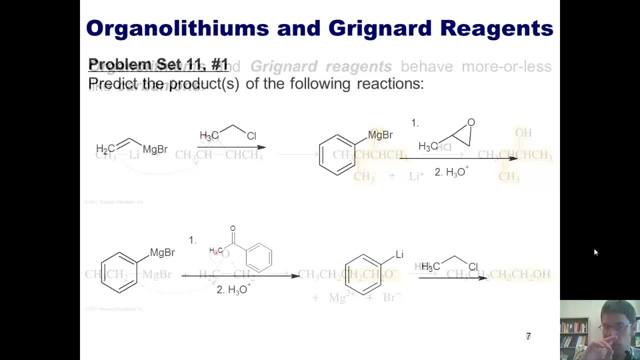 has been added on to this CH2 group. The negatively charged oxygen can then be protonated during an acid or water quench to give me this alcohol. This brings me to this set of problems. I want you to predict the products from the following reactions. 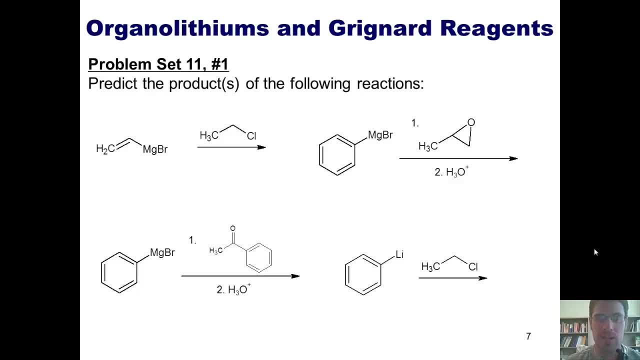 If you want to, this would be a great place to pause the video and attempt these on your own. first, because I'm going to show you the answers momentarily, Let's begin by taking a look at our first example. I have this molecule which is called vinyl magnesium bromide. 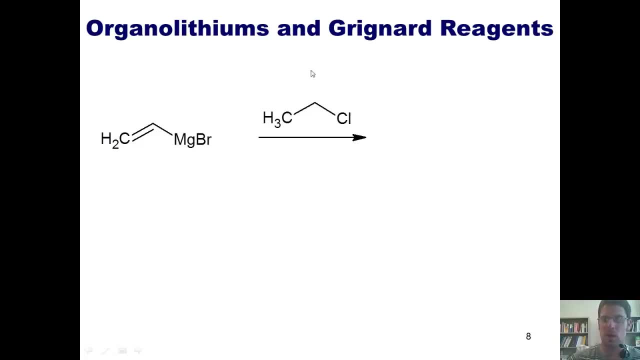 It's a Grignard reagent reacting with this molecule, ethyl chloride. Before we begin, I'm going to go ahead and number the carbons in both my starting material and my reactant, just so that we can keep things straight. 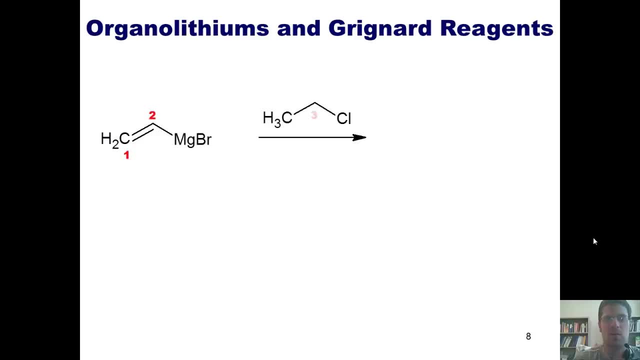 I've numbered them as shown here: One, two, three, four. You'll see why momentarily Now. as I've stated before, the carbon that's bonded to the magnesium is much more electronegative than the magnesium. Thus this carbon- carbon 2, behaves more or less. 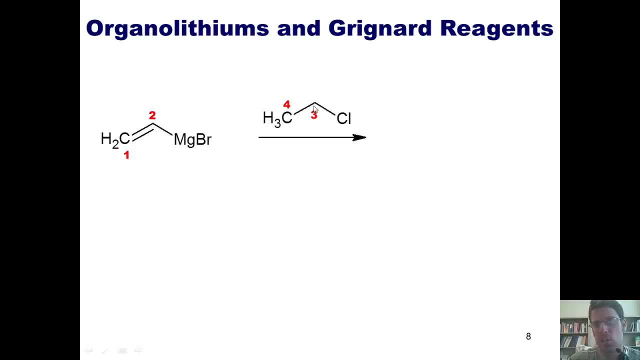 as if there were a negative charge on it. You'll note that over here, this carbon carbon 3, is bonded to chlorine, which means that this carbon has a partial positive charge. So what in the world happens when you react these two molecules together? 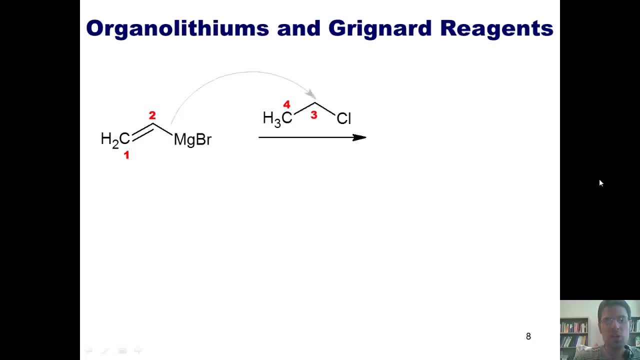 The negatively charged carbon, carbon 2, pushes its electrons, as if a nucleophile, into carbon 3 and kicks off this chloride. There's a bond then formed between carbon 2 and carbon 3, which ultimately forms this product. I'll let you take a moment to look at that to make sure that it makes sense. 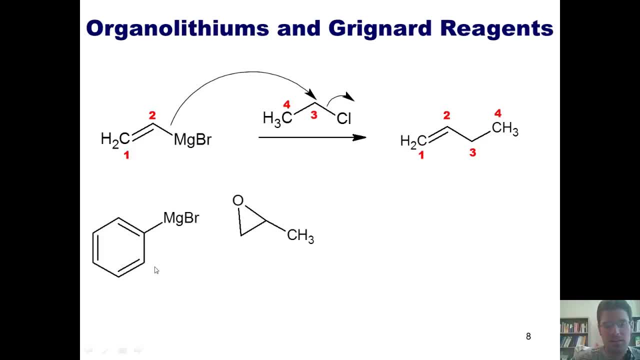 Here's another example. I've got my Grignard phenyl magnesium bromide reacting with this epoxide. Once again, I'm going to number my carbons: One, two, three in my epoxide as shown here. As I've stated before, the carbon right here in the ring. 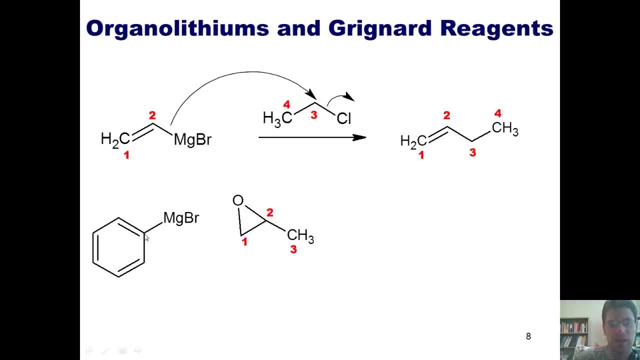 that's bonded to the magnesium behaves more or less as if there's a negative charge on that carbon. This negatively charged carbon then reacts as a nucleophile and, of course, is going to attack one of these two carbons in the epoxide. Which one is it going to attack? 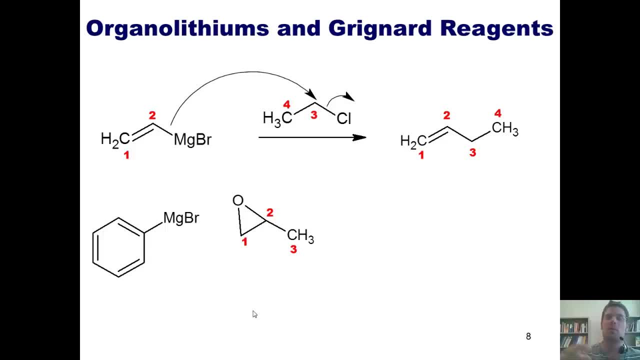 Carbon 1 or carbon 2?? Well, you might remember from our previous chapter that I said that nucleophiles, under basic conditions, attack the less hindered carbon in epoxides. If this were acidic conditions, then it would attack the more hindered carbon in the epoxide. 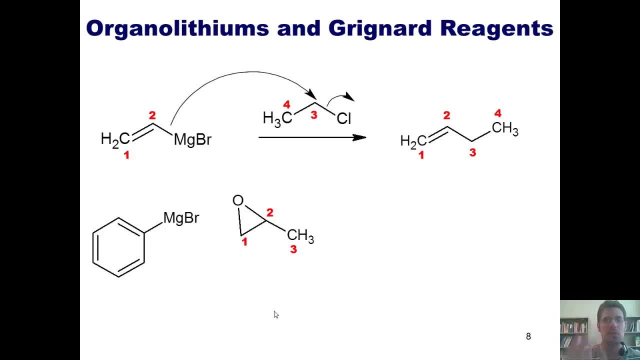 I should mention, by the way, that Grignard reactions can only proceed under basic conditions, Otherwise you would just attach a proton to this carbon. Thus, this carbon takes its electrons and reacts as a nucleophile, pushing into carbon 1 to form a bond with it. 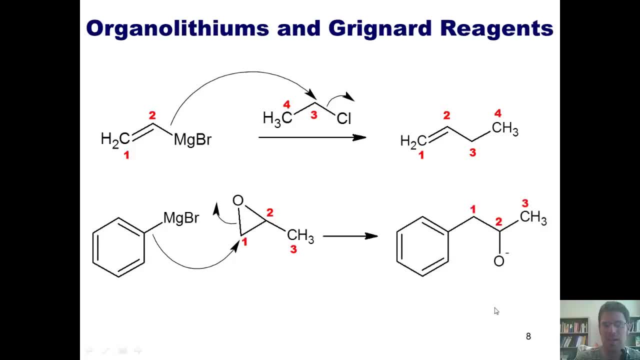 and pumping these electrons up onto the oxygen to give me this intermediate. You can go ahead and pause here and make sure that all the carbons and where they are located in the product makes sense to you. Now, of course, this type of reaction, as with all Grignard reactions, 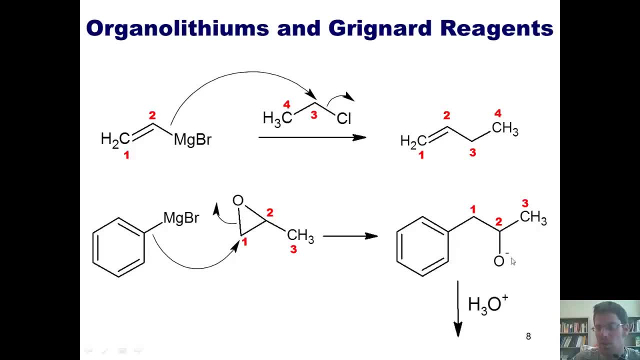 is quenched with acid or water. This will protonate this O- and turn it into an OH, which will be my final product. Let's take a look at our organolithium examples. I've got my phenyl lithium here reacting with ethyl chloride. 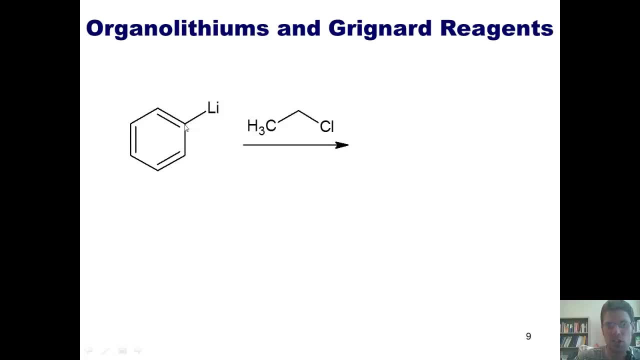 Once again, there's more or less an effective negative charge on this carbon. in the ring, There's a partial positive charge on this carbon attached to the chlorine and for the sake of keeping track of stuff, I'm going to number those carbons 1 and 2.. 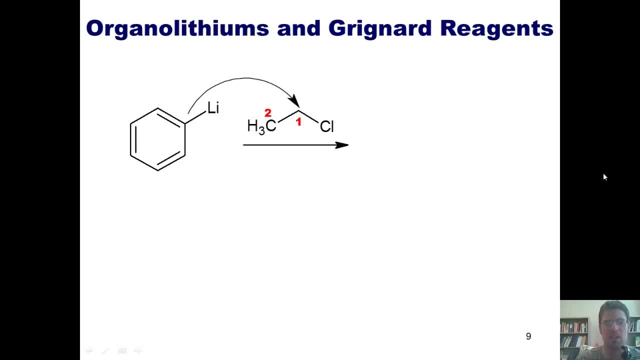 The negatively charged carbon, right here bound to the lithium, thrusts its electrons down into carbon 1, kicking off the chloride, and gives me this product right here. You can pause it and look at it and make sure that it makes sense. 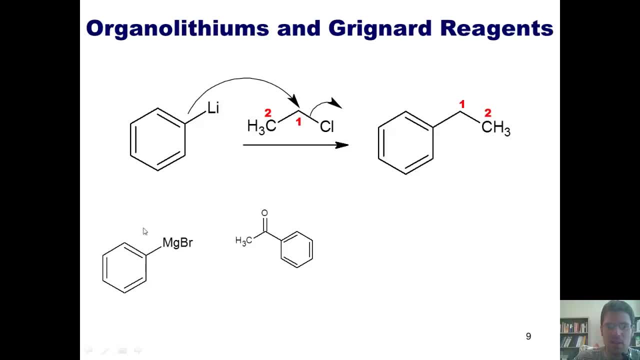 And here's my last example. This one's kind of interesting. I have once again a Grignard reagent over here. This carbon, attached to the magnesium, more or less behaves as if there's a negative charge on the carbon. It is an attacking carbon. 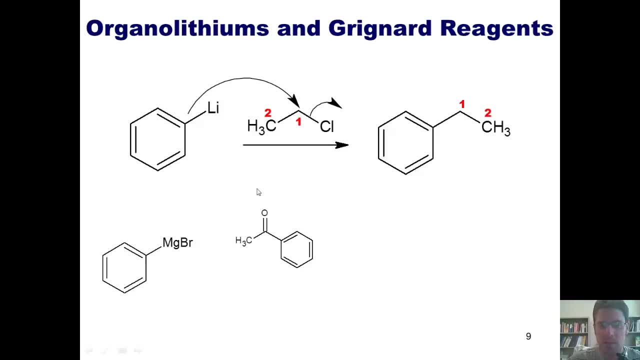 For the sake of keeping track of stuff, I'm going to number the carbons in my reacting partner over here: 1 and 2.. You'll notice that this carbon 1 right here, bonded to an oxygen, has a partial positive charge in it. 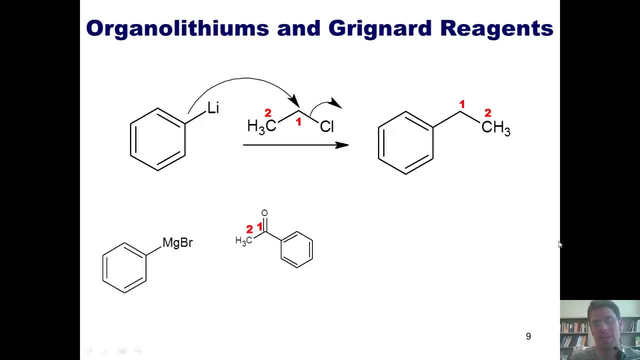 What is going to occur next? The negatively charged carbon in the Grignard reagent is going to come in here and form a bond with carbon 1, and as it does so, it's going to push these pi electrons up onto that oxygen. 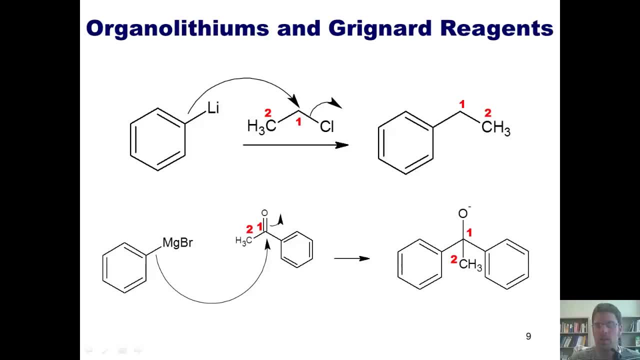 which gives me this intermediate. Once again, I've numbered the carbons 1 and 2, in this intermediate so that you can see where they started at This negatively charged oxygen will then get protonated when we quench the reaction with acid or water. 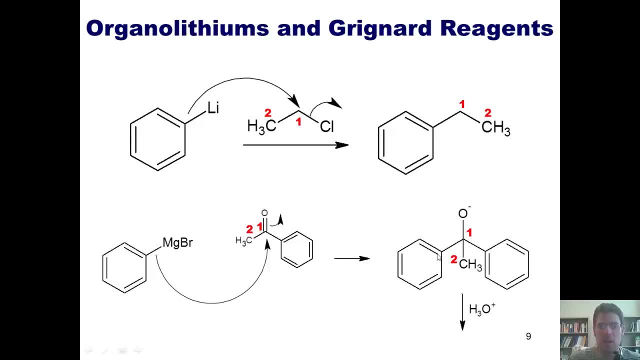 to give me an OH at this position. Now, this type of reaction right here might look a little bit scary to you guys at this point. I hope not, but if that's the case, please don't worry too much about it. Try your best to understand it. 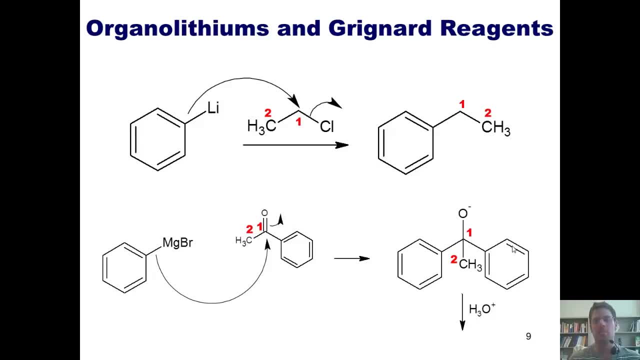 and recognize what's happening here And keep in mind that we're going to cover this type of reaction in extensive depth for the first three chapters that we cover during our semester 2 lectures on organic chemistry. Alright, that is the end of this lecture. 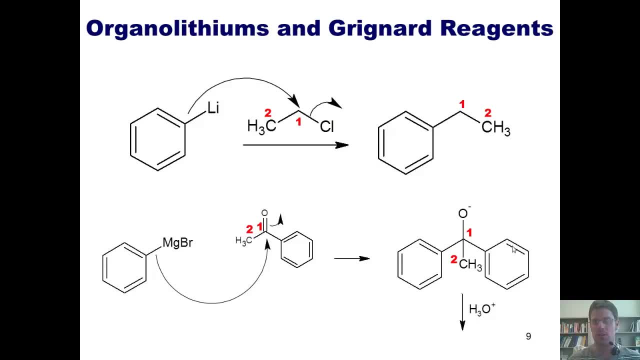 introducing you to organolithiums and Grignard reagents. Please stay tuned to my next lecture, in which I continue covering organometallic reagents and reactions. Until then, have an enjoyable rest of your day. 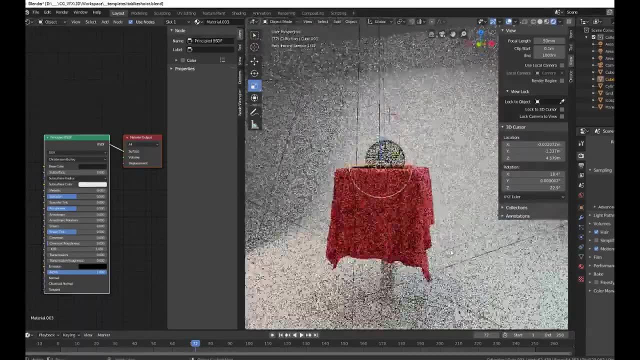 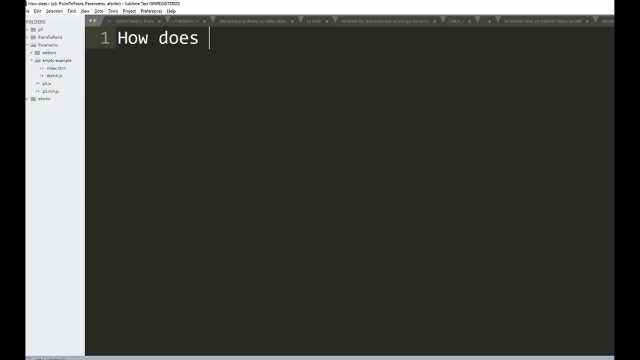 Oh, rendering- the most satisfying part when easing the render button. Have you ever wondered why rendering takes so long? Today we're going to take a look at how does rendering actually works. We're going to take a look at offline rendering and not real time, So every 3D scene has some 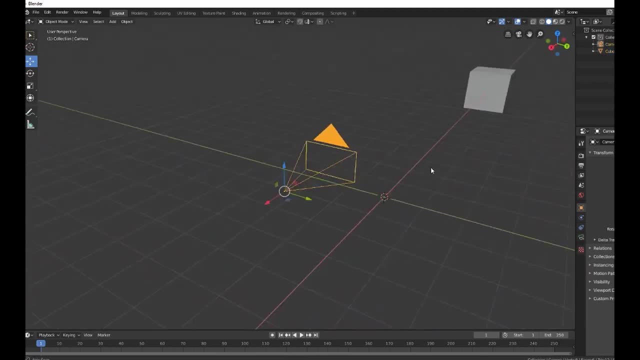 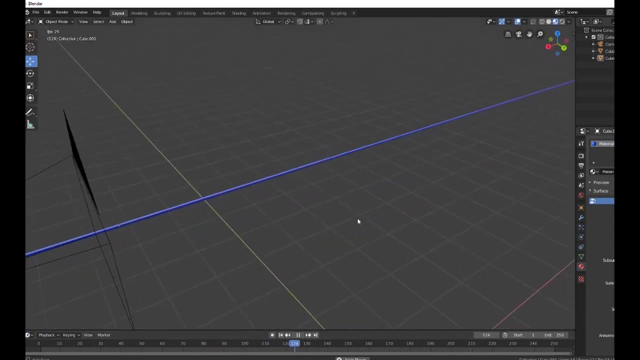 objects and a camera. The camera will be what we will use to actually render. a frame or an image has a render, The camera has basically a position in space and therefore here will have a cube rendered to it. We send to each pixels of the camera some rays. 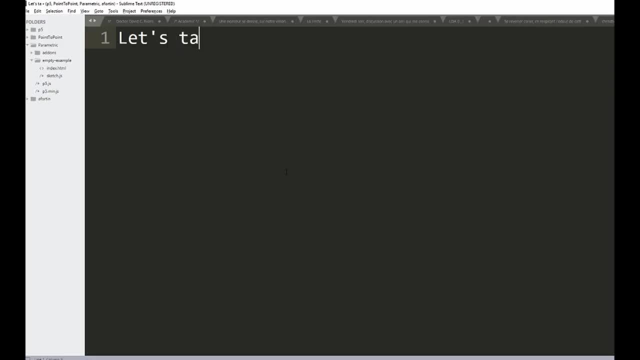 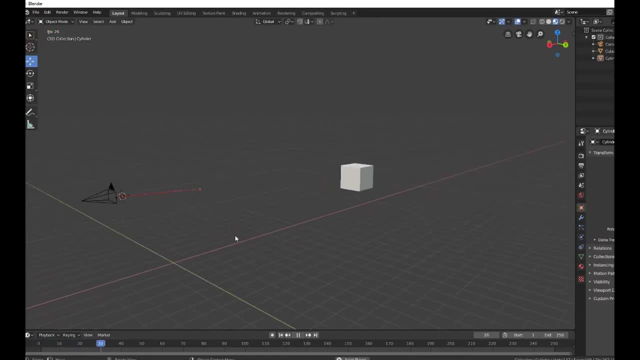 Here in blue, the rays is basically colliding to infinity. Let's take a ray that intersects with an object. That means that you send the ray in red right here and eventually the ray will collide through an object in the scene, here being the cube. 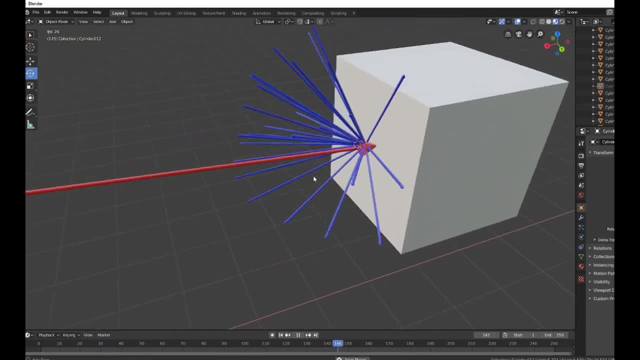 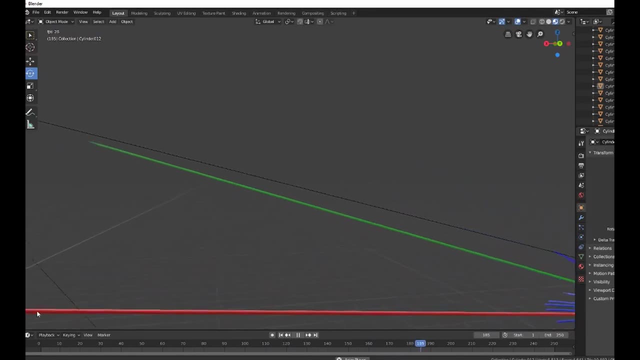 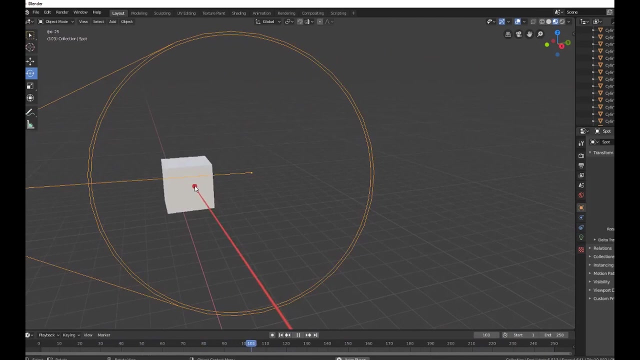 For every pixels you send the ray, and when a ray hits an object, you will send bunch of other rays, mostly in the shapes of hemisphere. All of those sub rays needs to hit a point when a light source is emitted. Here is a light source- then we intersect with a cube and send bunch of rays and